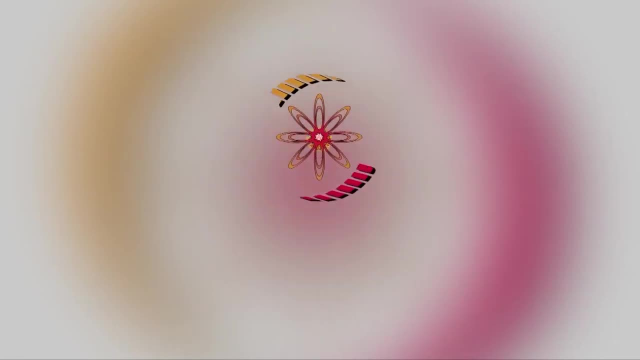 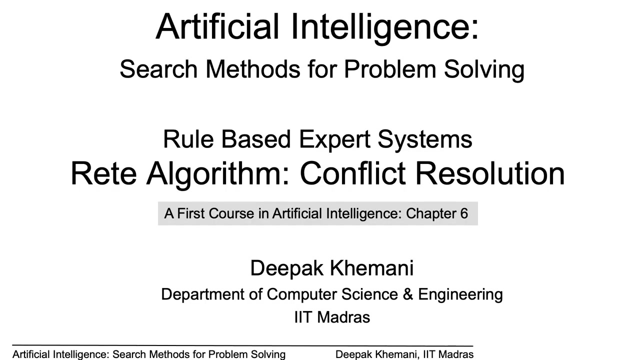 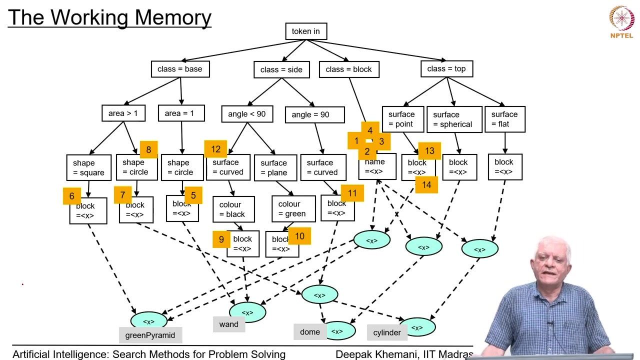 So here we are. This will should be the last lecture on rule based expert systems and the data net. We will wind up with some more examples and a small exercise for you to do. In the last class we were looking at this: four objects- the green pyramid, the wand. 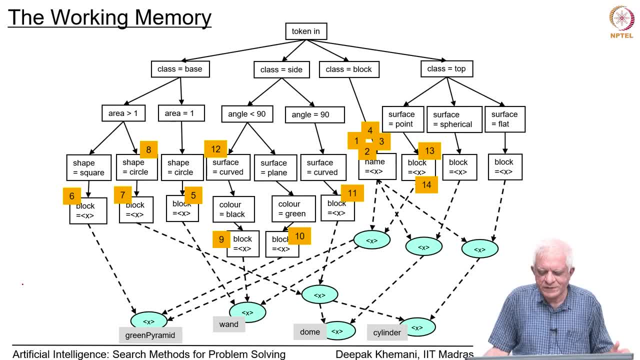 the dome and the cylinder And we had seen fourteen pieces of data And once you insert those fourteen pieces of data, then they go and sit in the working memory at some location. You can see that there were four blocks and all four of them have come and sit in this. 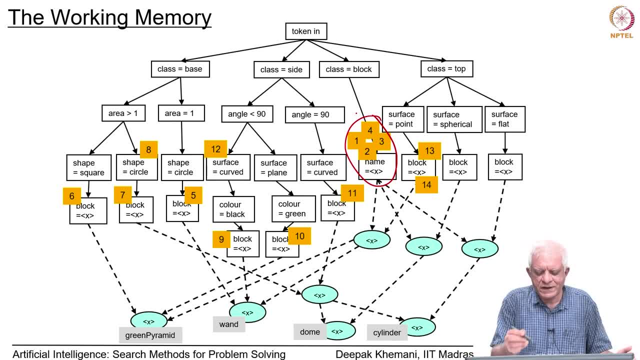 node here, because that is all it is saying: block and what is the name of the block? The name is a variable. There are four tokens sitting here, one with a value. whatever the values are 1,, 2,, 3,, 4,. I think What I have written here is not the value of the attribute. 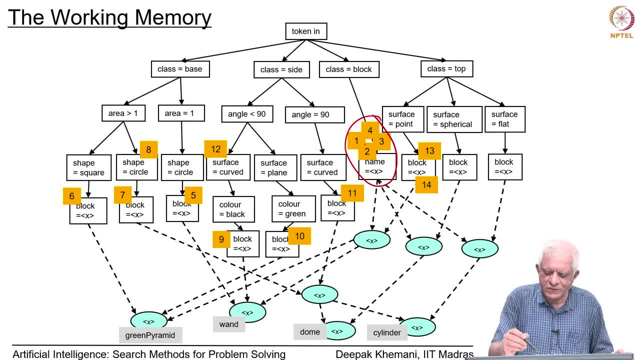 x, it is the time stamp of the token. So these values are all So obviously they stand for those particular tokens And you can see that this is where those fourteen tokens are sitting. And therefore the data network not only embodies all the 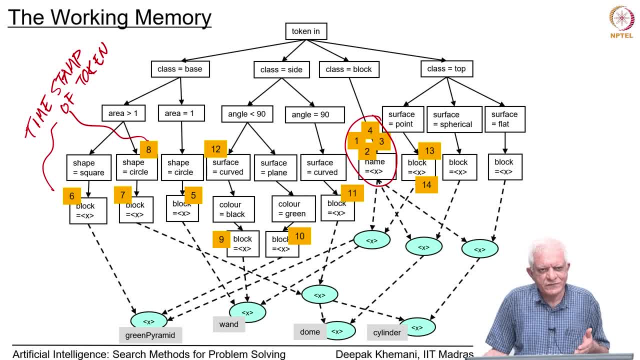 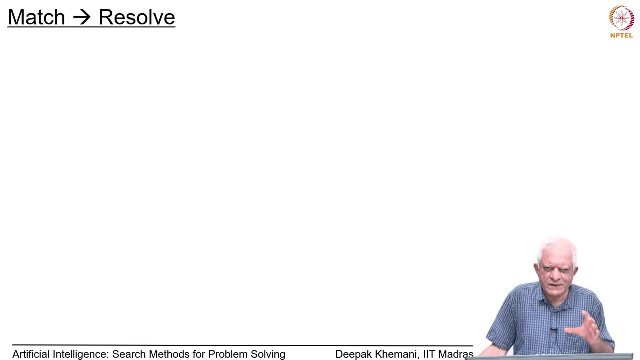 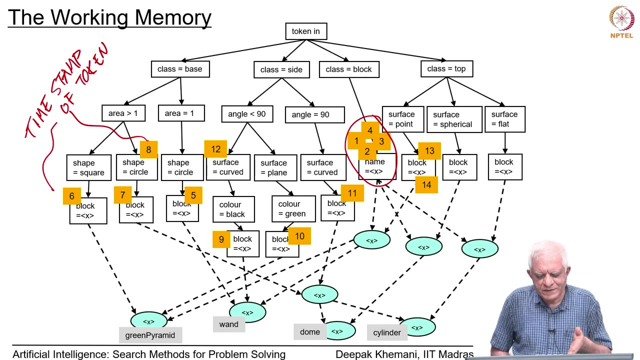 rules in your rule base system. it also serves as a memory for your rule base system, So everything is in one place here, essentially. So let us look at conflict resolution now. So, after you have done the match, which is what we have seen here, you have these fourteen working memory elements and two of these. 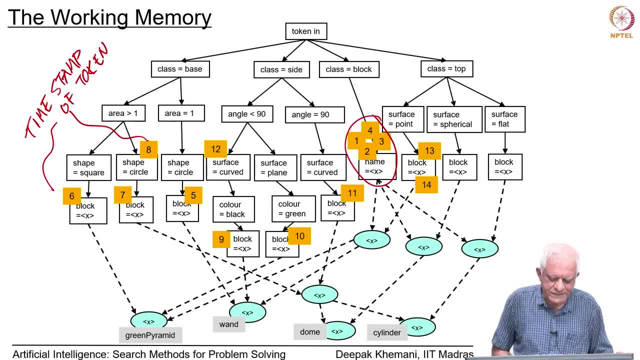 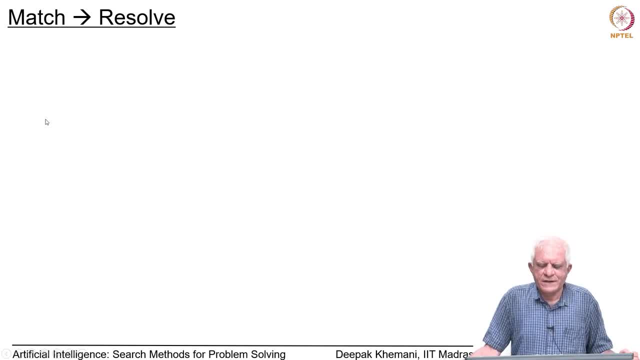 four rules: One is for the control right, the other is the control left And the other for matching. if you have done that little bit of exercise, which of those two should you select? And that, in general, is the task of conflict resolution in the second of the three steps. 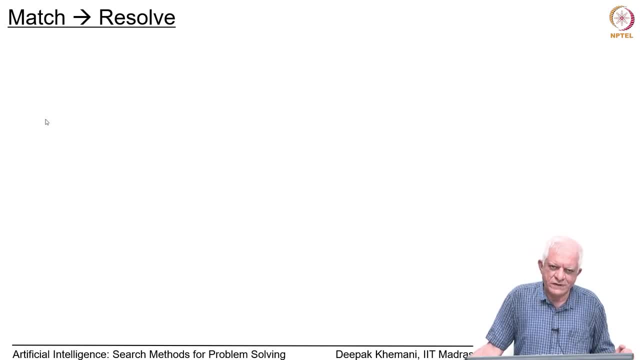 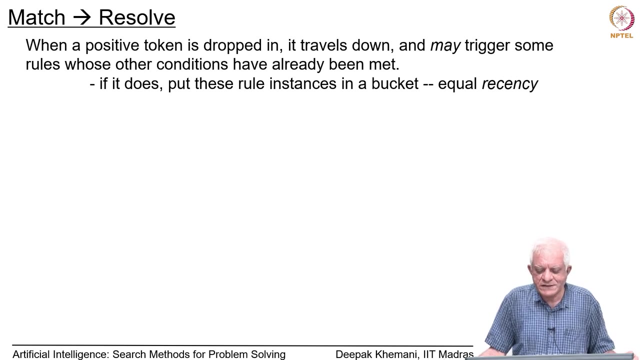 in the cycle: match, resolve, execute. How do we do resolve? So let us look at the different cases. When a positive token is dropped in, it travels down and it may trigger some rules whose other conditions have already been met. 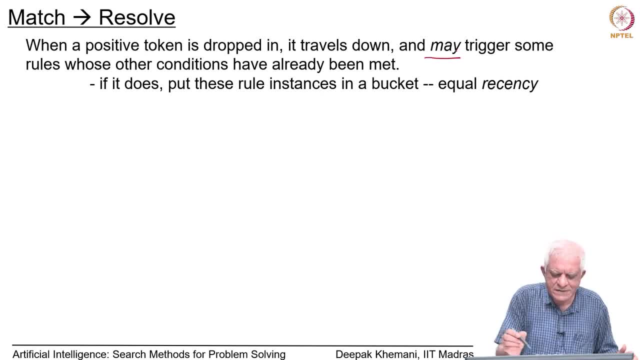 So that is why we say may trigger, because if it is one of the many patterns, it has to wait for other conditions to be met. If the other conditions have already been met, then this is the last piece in the jigsaw puzzle. 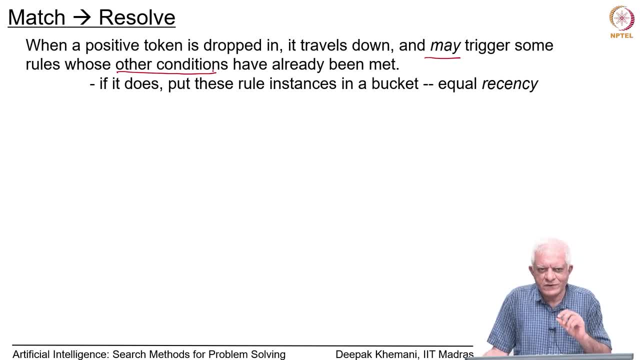 So that is the rule, as you might say- for that rule to become active, or more than one rule could also become active at the same time. So when you drop a token and it triggers some rules, or one rule, or more than one rule, 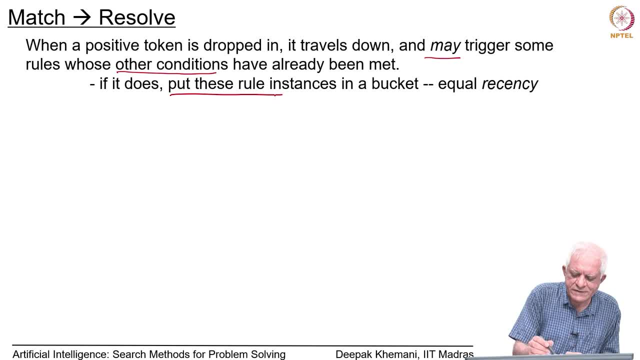 then we can put all these rules which instances right. remember that we are always talking about rule instances, rules plus timestamps of the data which is matching. That is the element in the conflict set. We can put all these rule instances in one bucket and we know that all these rules have. 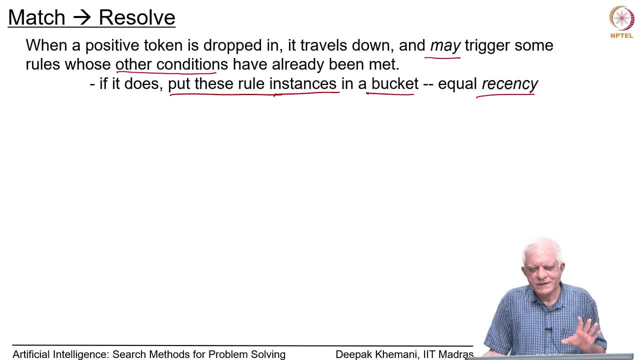 the same recency. In fact, it is the highest recency because this is the last working memory element you dropped into the system and it triggered some rules. So if you are going to be using recency strategy, then one of these rules will be selected by 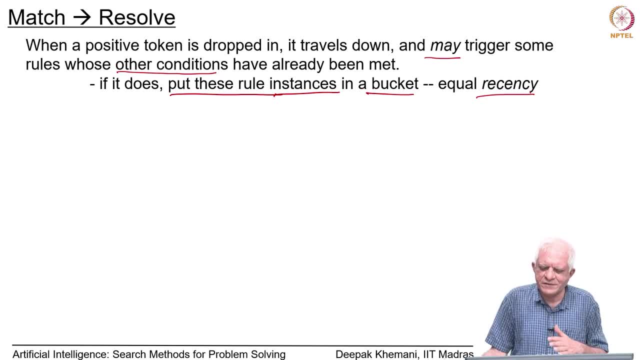 conflict resolution And other rules may have matched earlier, but they are waiting somewhere. So this is how to implement. recency is that the moment a rule gets triggered, you put it into a new bucket and that new bucket tells you that these are the rules with the. 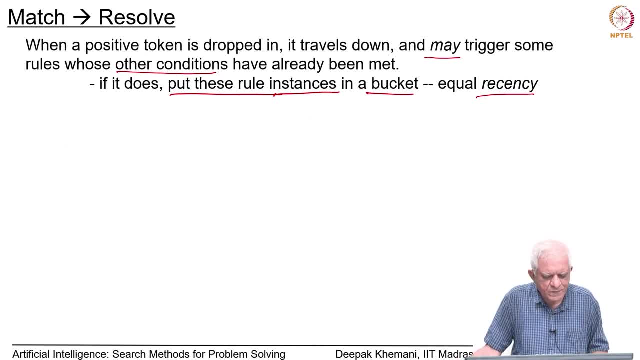 most recent working memory element. If you want to talk about specificity, which is the other major conflict resolution strategy that we had seen. 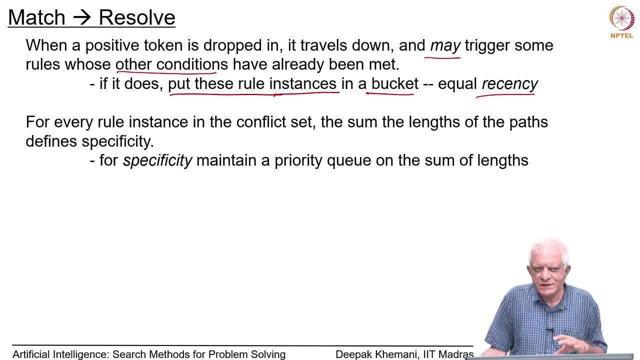 Not a lot of trials yet I receive. These rules have to be defined by the number of tests that a rule does before it matches. 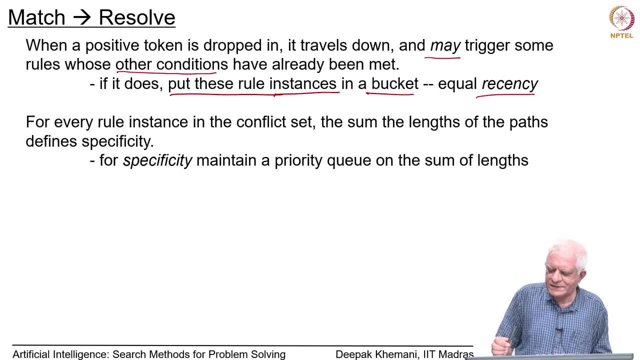 essentially, and the number of tests, as you can imagine, can be approximated by the sum of the lengths of the paths. Remember that if the Green Parameter Rule, for example, had four patterns, it needed four working memory elements to the place and each of those four working memory elements. 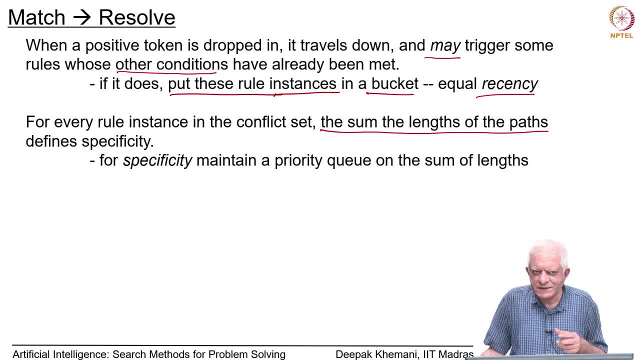 travel down some path in the written network, The length of that path is indicative of the number of tests that are being done by that particular rule. essentially So, if you just add up the lengths of the paths, then you would have a measure of specificity. 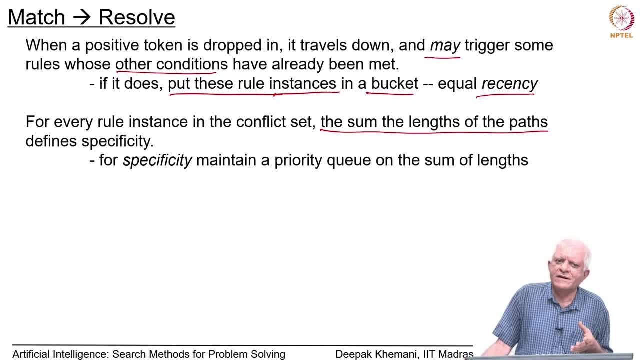 of that rule. So remember, the property of specificity is only a property of the rule. Recency data depends upon the data. which data was the last one to be inserted? Specificity simply looks at all the rules and says that of the rule instances that we 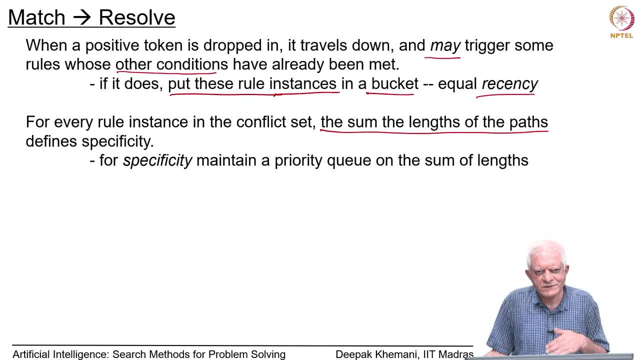 have. this is the most specific. It can say that simply by looking at the rule, because you just look at the paths which lead up to that rule, add up the lengths and you have specificity. So if you want to use specificity as a strategy, you can just maintain a priority queue on. 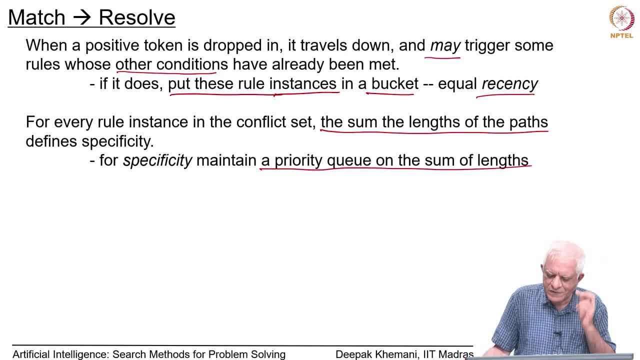 the sum of the lengths of this thing and keep taking rules along this thing. So the two major strategies have been taken care of here. Now we will move on to the next slide. Now, remember, at the end of the last lecture we said that the key point about the RETA 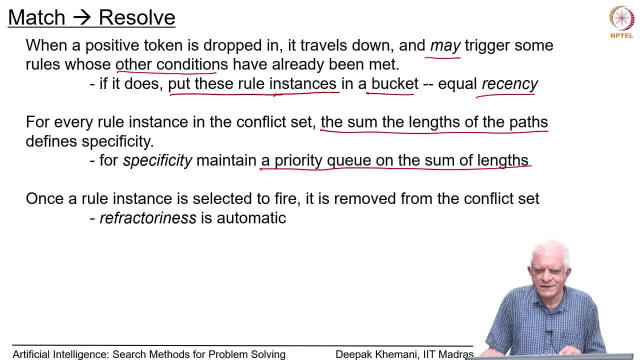 algorithm and the RETANET is that every working memory element is inspected or seen only once. essentially So it goes down the network and it may trigger some rules. essentially So a rule instance now lies in the conflict set. You can implement the conflict set as a priority queue or whatever the case may be. 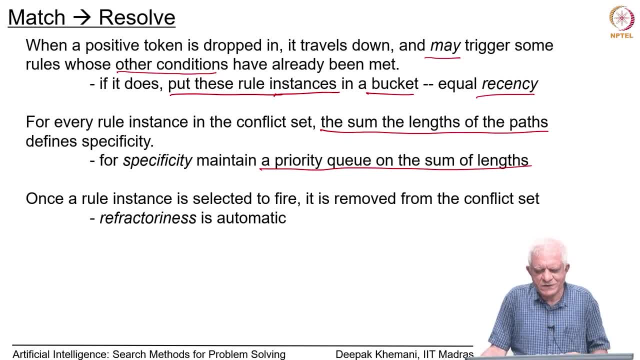 It will be a priority queue in any ways, Whether it's recency or specificity or whether it is MEA, then it has to be a slightly more complex data structure. But once a working memory element triggers a rule and the rule goes into a conflict, 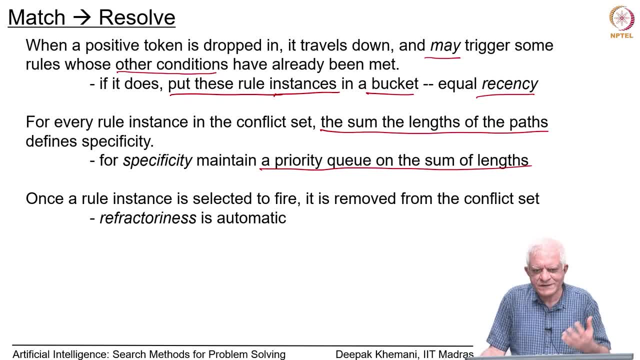 set. it's lying there. It's like a fruit, in some sense, which has ripened in a tree. essentially, It's waiting to be plucked and eaten, or executed, as the case may be, Okay, But like a fruit that you can eat only once, a rule can also be only plucked only once. 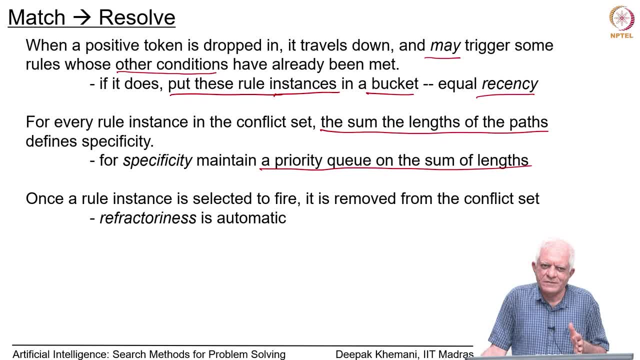 You can remove it from the conflict set and execute it, but then it's no longer in the conflict set And therefore the property of refractoriness that we were interested in is automatic. So, irrespective of whether you are using recency or specificity, refractoriness is taking care. 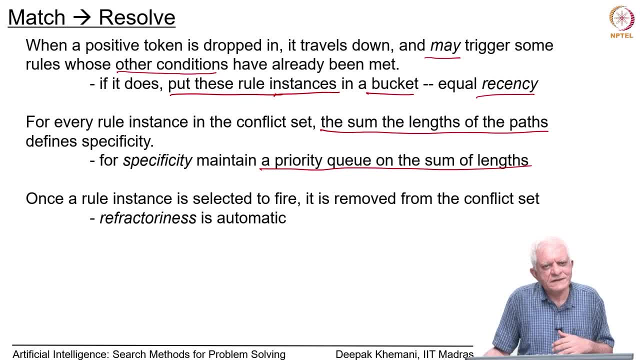 of the fact that you will remove the rule from the conflict set at the point when you execute it. So that takes care of that. Then what about negative tokens? If you drop a negative token? remember that a negative token is generated whenever the 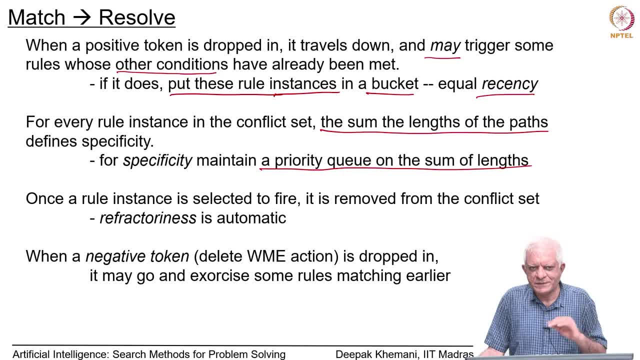 action. part of a rule says: remove this working memory element or delete this working memory element. and delete or remove is also part of modify. If you want to modify a working memory element, it is equivalent to saying remove the old element. 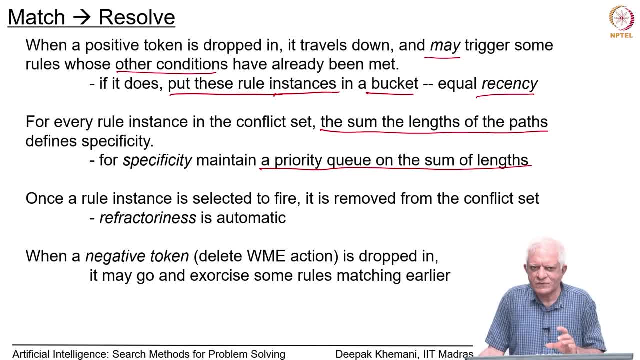 And replace it with a new one. So remove is the negative token, which is generated either by the remove action or the delete action, depending on what you want to call it, or by the modify action, essentially So, once a token is generated, you send it down. 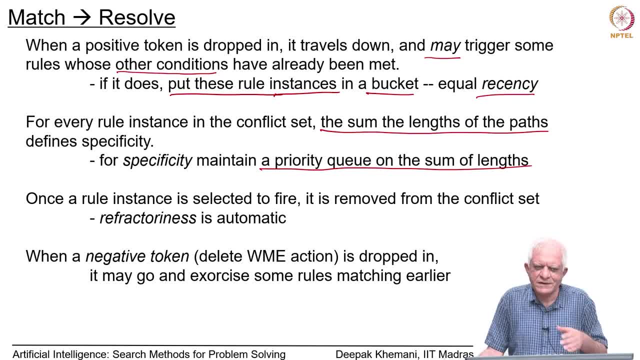 What is the task? You want to delete it from working memory. So obviously the data network, the alpha nodes, will guide that token down to where it was lying, And once it lies there, then you would know. So delete it from there. essentially. 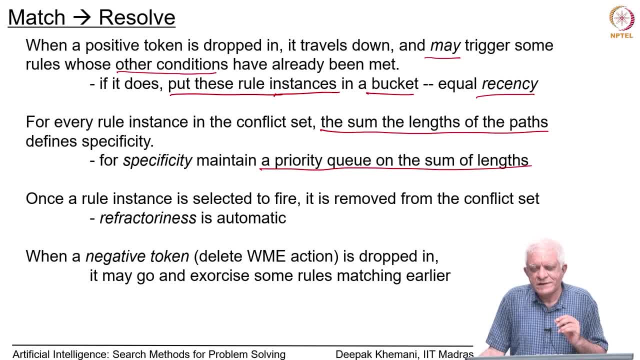 Taking care that if you delete a token, then if there was some other rule which was matching this token, you have to be careful to remove that other rule from the conflict set as well. essentially, So this is something that you have to do if your system has to be correct. essentially, 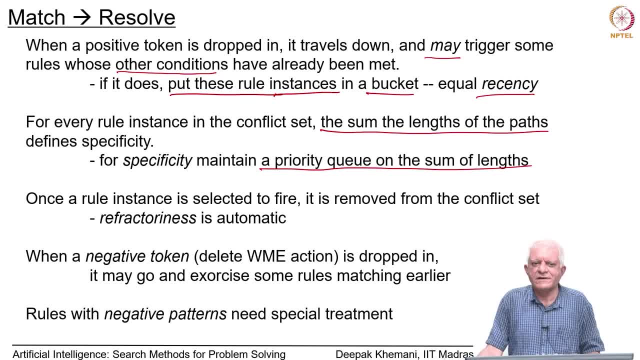 The last thing that we have not spoken about too much is negative patterns. Remember what are negative patterns? We talked about ranking, assigning ranks to students. We said that if there is a student with marks M and there is no student with marks more, 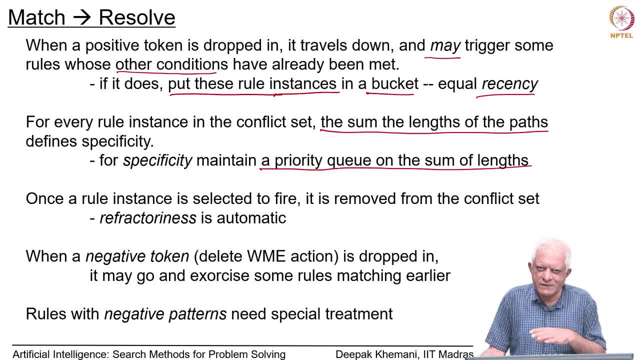 than M. this pattern, which said that there are no students with marks more than M, was a negative pattern. essentially, which is different from a negative token? A negative token talks saying that remove this working memory element. Negative pattern says there is no such working memory. 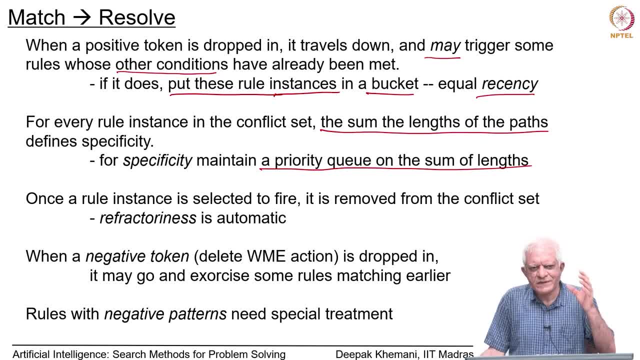 Okay, How do we handle negative patterns? So whenever a positive token travels down a destination or a negative token travels down to a destination, a rule which has a negative pattern will be looking out for it. essentially, So, if a rule says that there must be no such negative pattern, and if a pattern arrives, 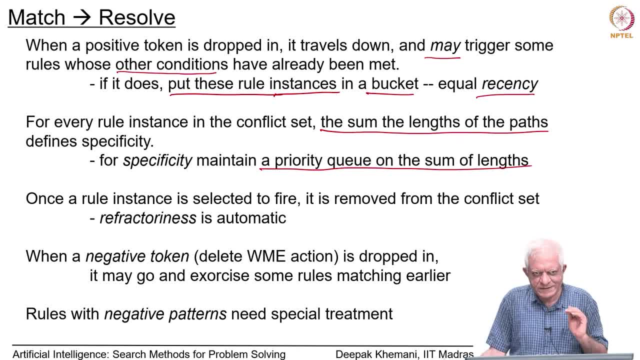 then it must be removed from the conflict set essentially. On the other hand, if a rule, if a negative pattern had come, a negative token had come and deleted something which was required not to be there by a negative pattern, then that 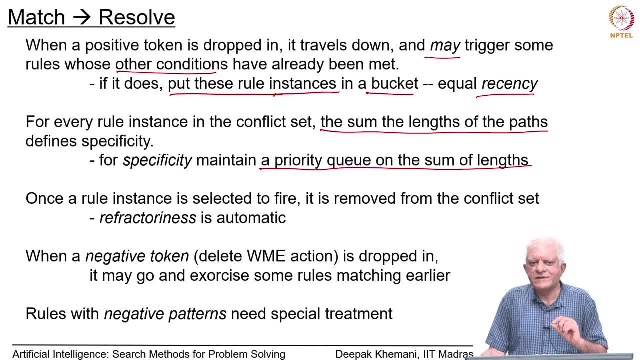 rule must be removed. Okay, Now activated and put it in the conflict set. Okay, So I have done this in a little bit of a hurry, but if you just think carefully about this, the fact is that it is a token which are travelling down and the pattern which is a negative. 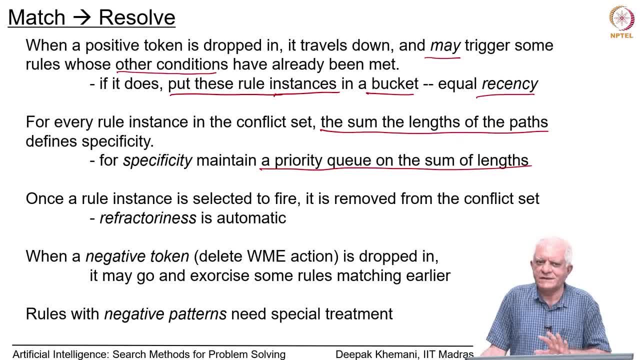 pattern says that. essentially it says that I do not want such a token. If such a token comes and if I was matching earlier, I will go out of the conflict set. but if a negative token comes and I was not matching earlier and it has deleted the token, 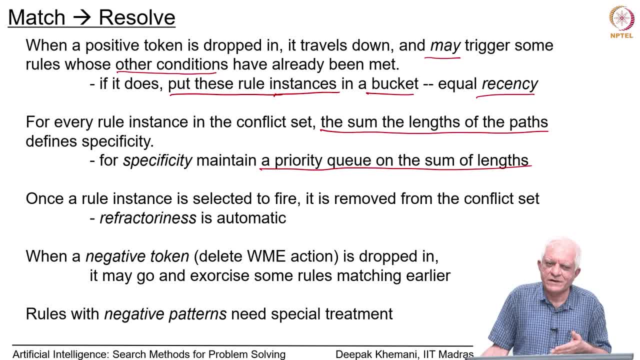 which I do not want. Then I should go into the positive, go into the conflict set. It needs a little bit of thought and hopefully you will work on it. Let us look at some examples more so that we get a feel of this whole thing about data. 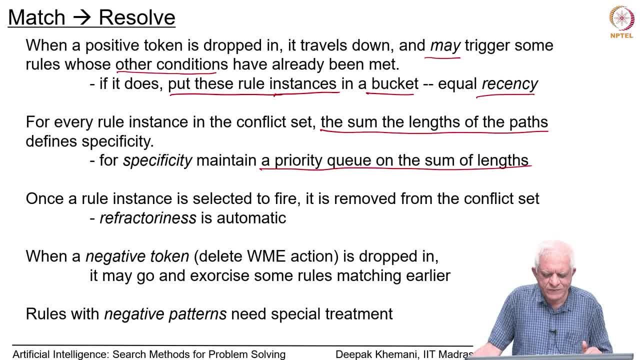 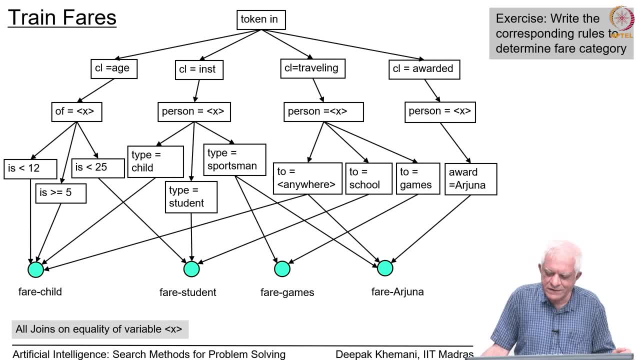 networks. These are some of the networks that we have worked with over the last few years while teaching the course. So here is a network. I have not written the rules. I will leave this as an exercise for you, But you can see that it is talking about train fares. 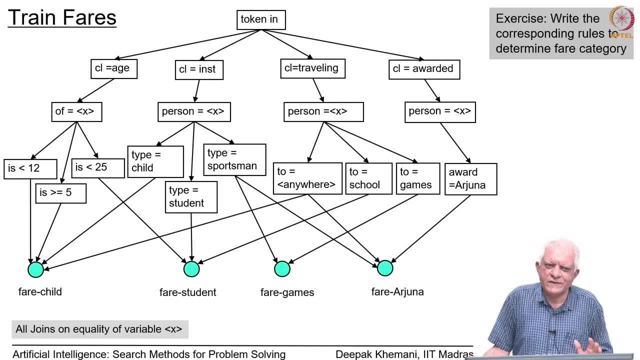 So in India a lot of times we get different kinds of concessions. We have to pay different kinds of fares depending on who we are, and so on. So, for example, students have concession if they are travelling to college and Arjuna. 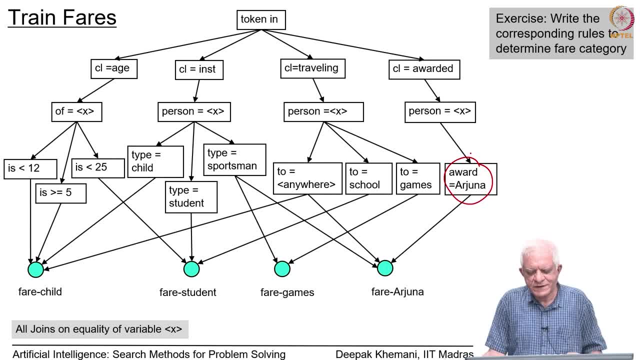 awardees probably get to travel to India. They are free, and so on and so forth. So I have not stated what the right-hand side of the rules are. I have simply stated that there are four rules here. One is: what do you pay for a child? what do you pay for a student, and under what conditions? 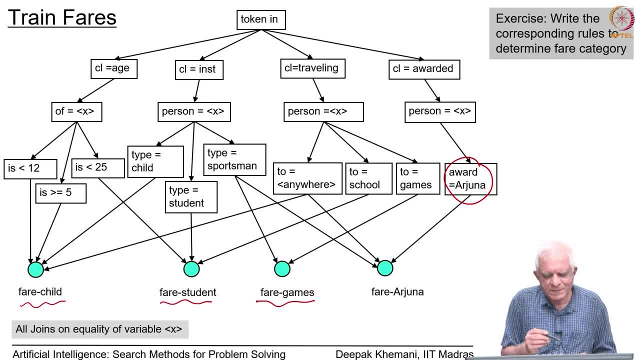 What do you pay if you are going to, let us say, take part in national games or something? What do you pay if you are an Arjuna awardee winner? These four rules have been kind of embodied into this network And I will urge you to try and look at this and try to write the rules which correspond. 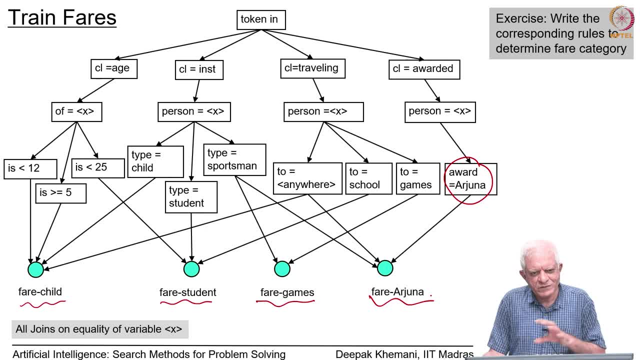 to this network. Remember that a network is equivalent to the rules. We are not talking about data here, we are only talking about the rules, essentially. So this is one such rule-based system which decides the fares- train fares as to how much. 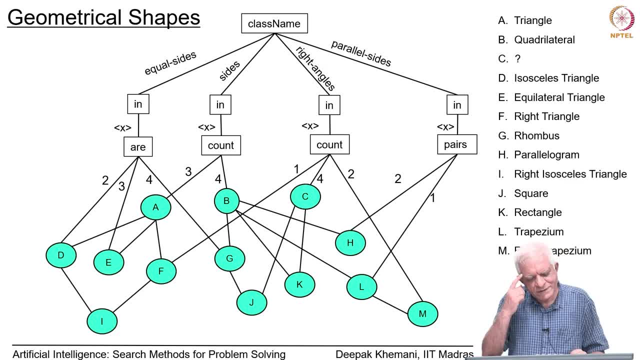 you have to pay. Here is another. There is a classification problem for geometric shapes, and the attributes that we are looking at is how many sides in a shape are equal, how many sides are there to start with? So we are looking at figures with three sides and figures with four sides. 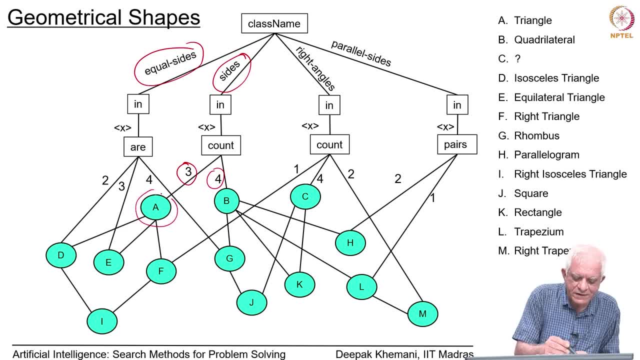 As you can imagine, figures with three sides are triangles. So you can see that A refers to a triangle. It is enough to say that something is a triangle if it has three sides, but there are other conditions. So, for example, rule F says that it is a right triangle. 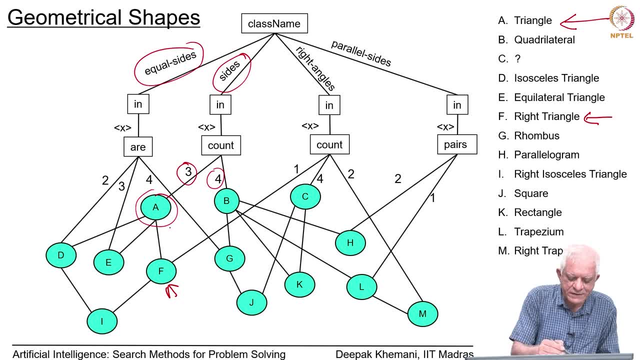 So it is a triangle, so one pattern has to come here, but it needs another pattern from here. So in this pattern it says how many right angles are there in the figure. So obviously a triangle can have only one right angle. and if that is the case, so if 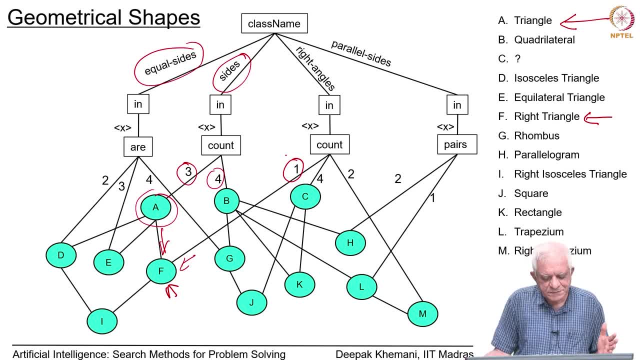 it is a triangle, and if it has a right angle, it has a right angle, then it is a right triangle, essentially. Likewise, you can see that this D is meant for isosceles triangles, and it says that the number of equal sides is 2, and if it has got three sides and two of them are equal, 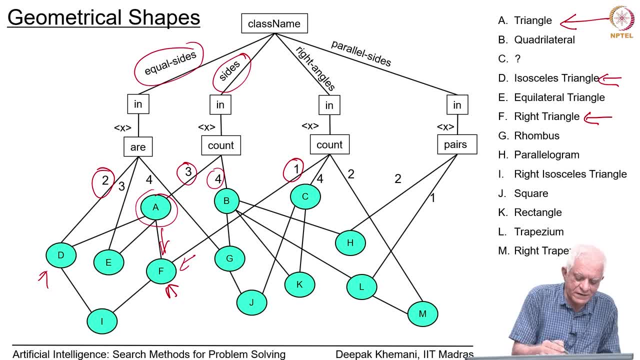 then it is an isosceles triangle. If it is an isosceles triangle and also is a right triangle, then it is a right isosceles triangle. So you have different rules for different things, and some of these things are mentioned. 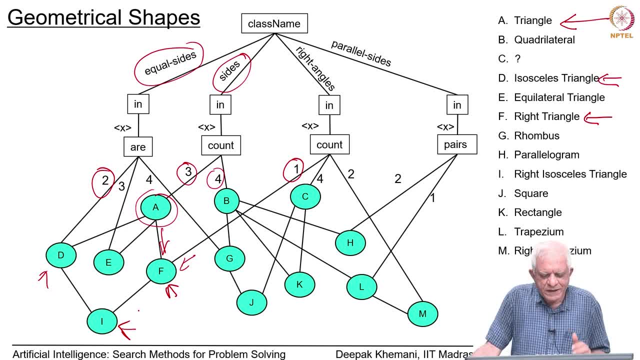 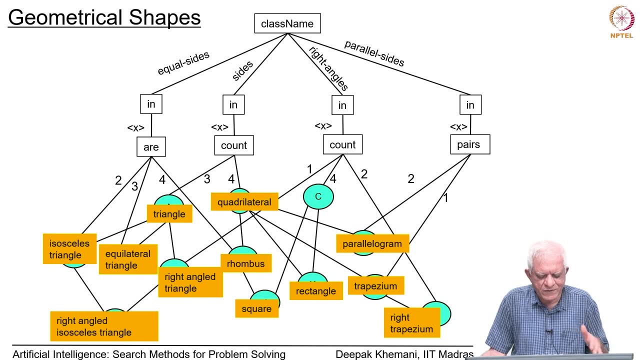 here Again. I would urge you to write these rules in an ops file language and see what your rule-based system looks like. This is another representation of the same diagram. here the names of the shapes are mentioned. The names of the shapes correspond to the rules that we are talking about. 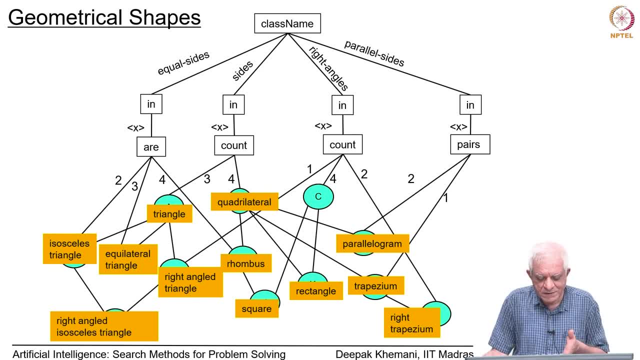 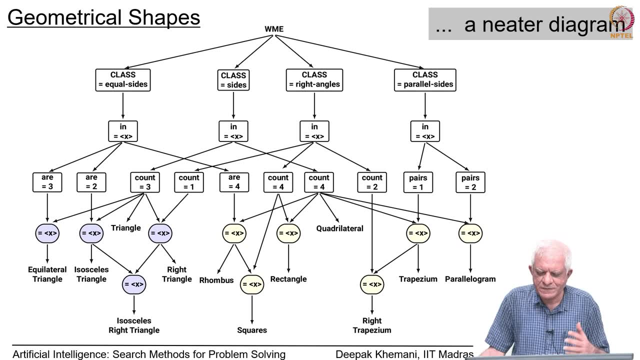 You can see that there are many shapes that we are talking about: parallelogram, rectangle, rhombus, square, and so on and so forth. And here is a neater version of the same diagram, thanks to my friend Pascalan, who has a tendency. 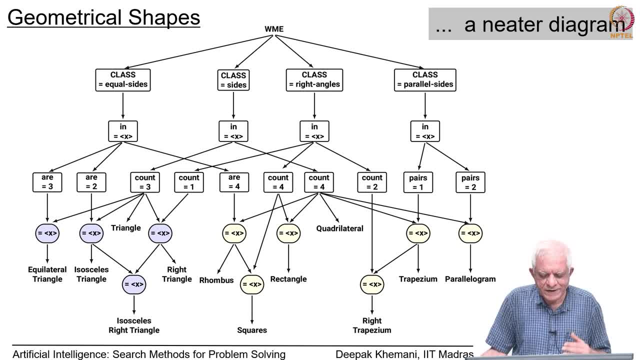 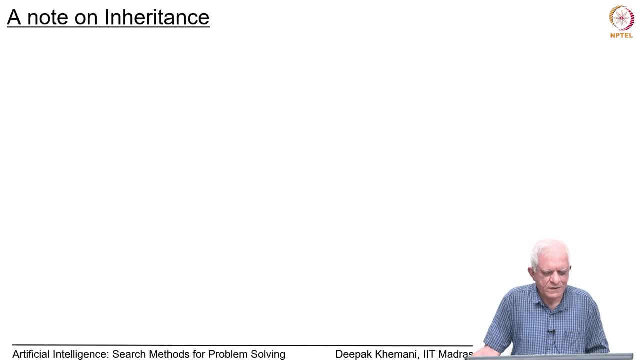 to spend a lot of time drawing neat diagrams, and this is one that he had produced some time ago, but it is the same data network. Thank you, Bye. Well, note on inheritance here, essentially So. inheritance is something, of course, we have not been speaking about in this course. 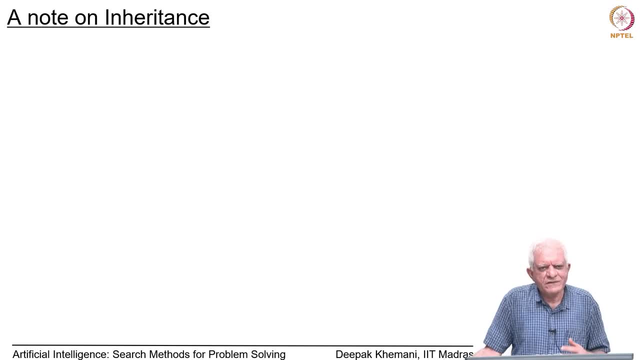 at all. We have been talking about search methods for problem solving and we have been trying to see how search is integrated into different kinds of problem solving activity, for example in rule-based expert systems. But just to mention in the passing, since we just saw this network, you can see that 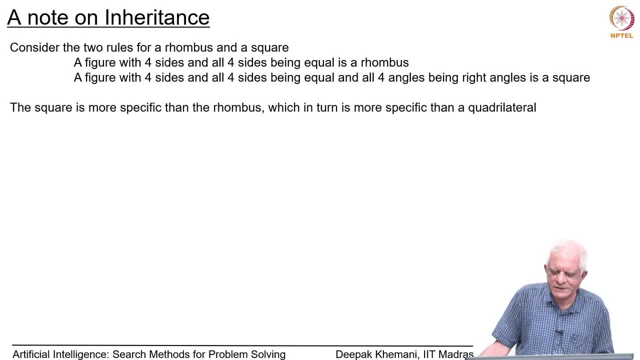 in the network that we just saw, There were two rules: one for a rhombus and one for a square. If you want to write those rules, then they would look like this: A figure with four sides, and all four sides being equal, is a rhombus, a figure with four. 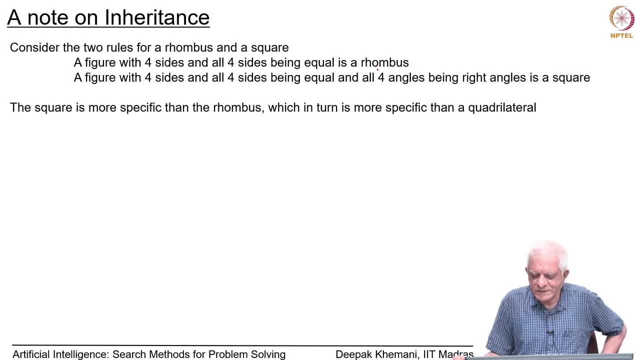 sides and all four sides being equal and all four sides being right angles is a square. Now I could have easily in some language, if I could describe it, I could have replaced this part Okay, And replace it by saying: a rhombus. a rhombus, with four angles being right angles is a square. 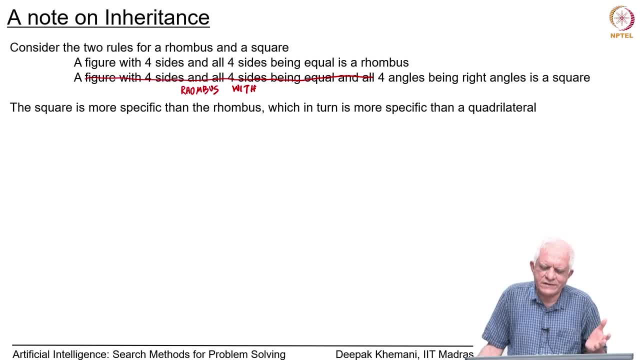 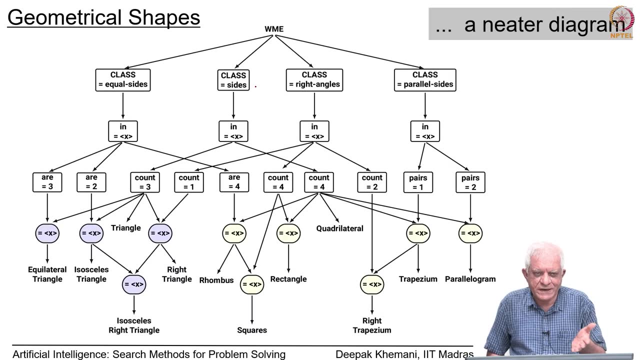 I could have said that as well, But of course, your how you express, how you describe a shape is dependent on the language that is available to you. In our case, In the rules that we just saw in the this thing we had, how many sides are equal? how? 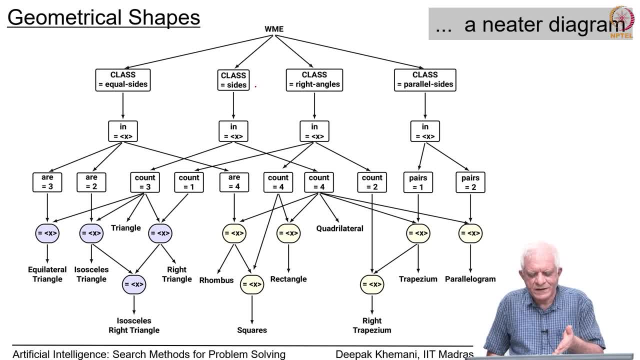 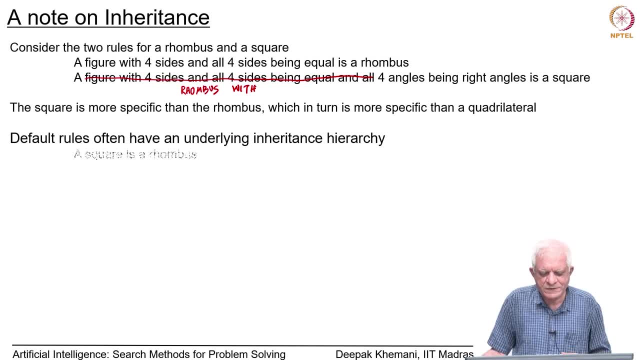 many sides does the system rule have and how many right angles are there? how many parallel sides are here? These were the attributes you are looking at, whether something is a rhombus or not, essentially, But in some language we could do that, and this has something to do with default rules. 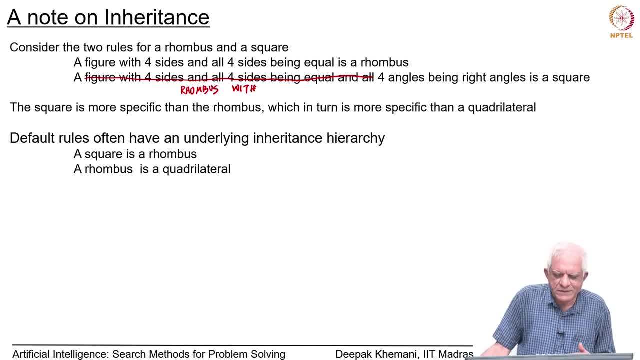 We have seen default rules earlier, But they also have an inheritance hierarchy: that a square is essentially a rhombus, a rhombus is essentially a quadrilateral, and so on. This happens because the quadrilateral rule is above the rhombus rule and the rhombus. 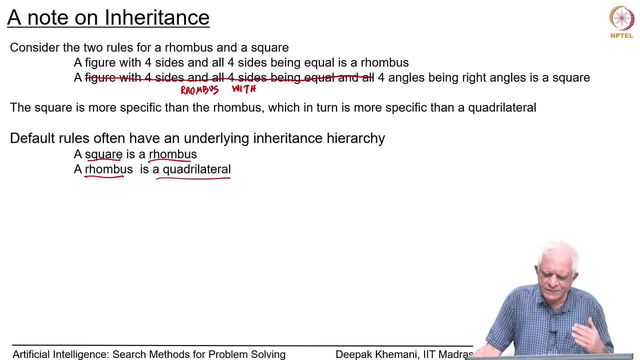 rule is above the square rule. Now, if you look at these kind of relationships, inheritance hierarchies, default rules and the subsumption relationship that a rhombus is a quadrilateral, can be expressed in logic and it is done. also, we are not doing too much logic here. we will do a little bit next. 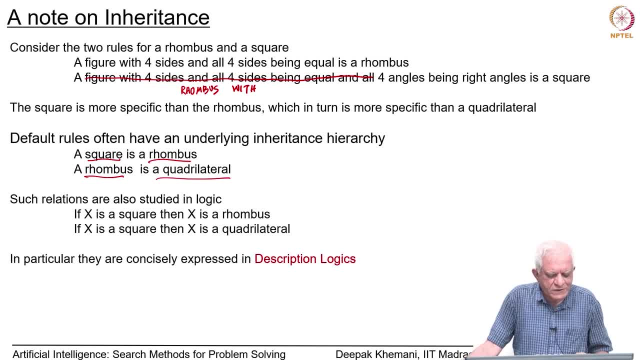 week. But we could have expressed it in logic and said that if x is a square, then x is a rhombus for all x. if x is a square, then x is a rhombus. Okay, If x is a square, then x is a quadrilateral. we could have said these things: 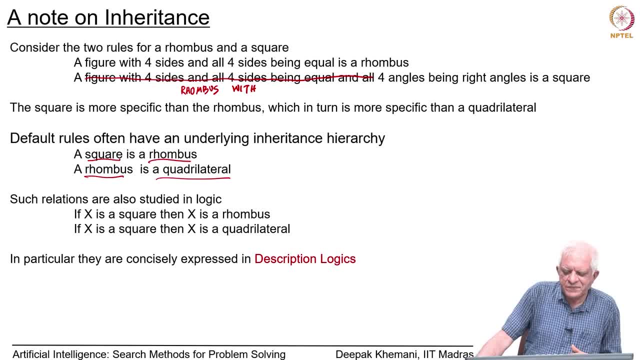 These things are done, actually very succinctly, in description logics, which are very popular nowadays because they are the basis of constructing taxonomies, and taxonomies are very useful when we do things on the internet, especially internet e-commerce and so on, And taxonomies are a part of many. 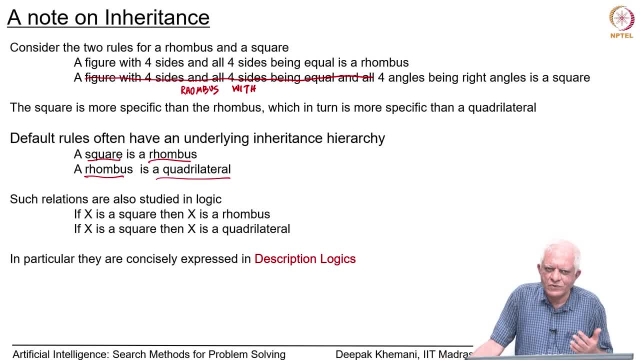 This web 2 and web 3 kind of applications. And there are these languages like OWL, which some of you may have heard, which are based on something called description logic. We will not have time to do that here, but I will do a little bit of a sales pitch and 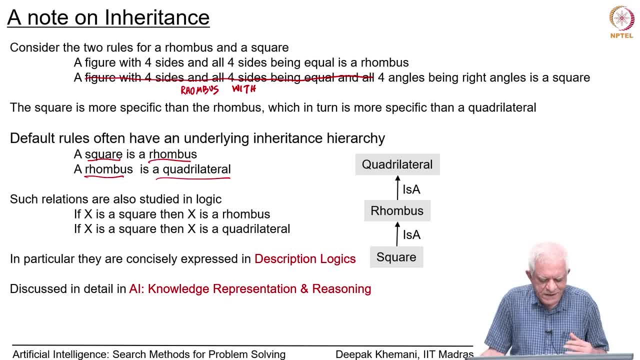 if you are interested, you should come to the course which is AI, knowledge, representation and reasoning, which is offered in the next semester, next offering There. So let us talk about relations like is a. so a square is a rhombus, a rhombus is a quadrilateral. 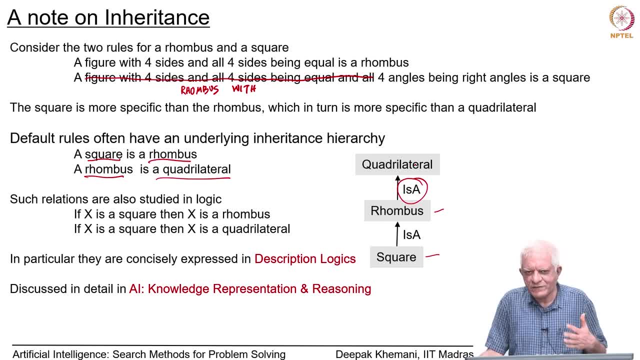 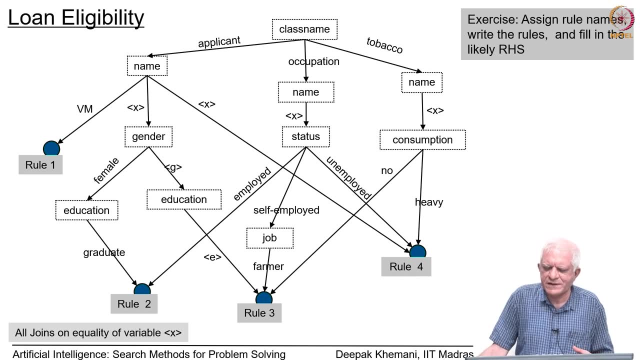 and so on. You can construct taxonomies and things like that, And these are languages to describe things, or noun phrases, languages for noun phrases, and they are called description logics. Here is one other example that I mentioned. I had said in the beginning that bank managers 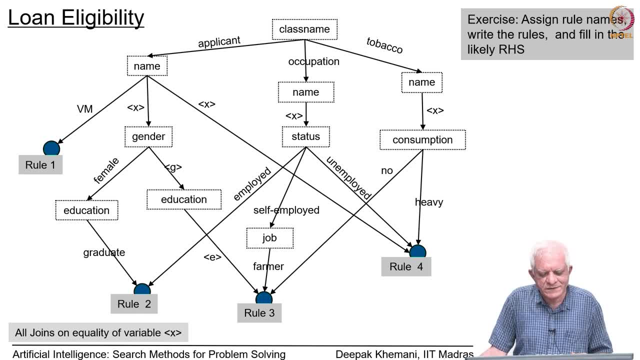 would often like to express their loan conditions in some succinct way and leave some system to take care of whether some applicant is eligible for a loan or not. So here is a small network we had constructed some time ago. Again, I would ask you to write down the rules for eligibility of bank loans. 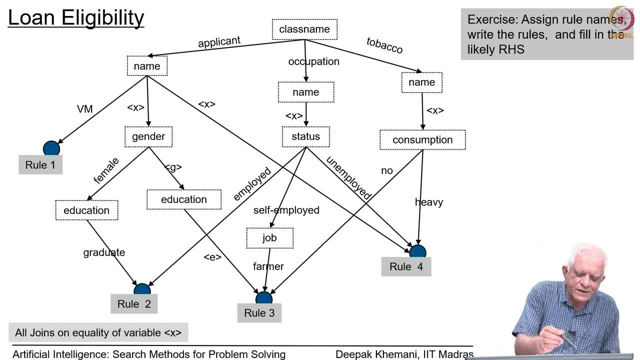 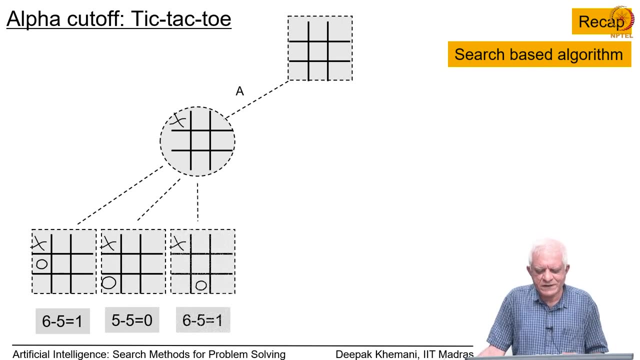 You might notice that in some countries, just having a particular name is enough for you to get a loan. Let us move away from classification. let us go back to games. you know that something that we looked at and this diagram is, repeat from the game playing lectures about how. 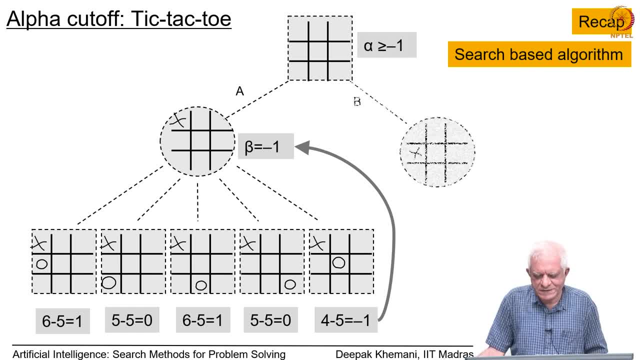 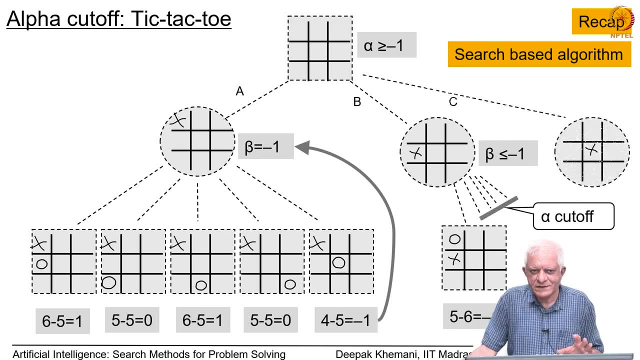 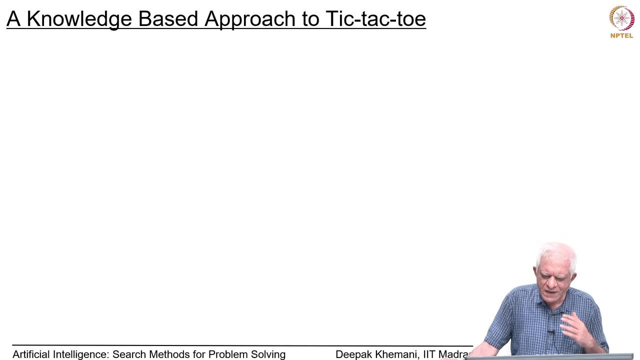 we can play games using alpha beta search and this was just illustrating that. we do not want to go into the details again here. just highlight the fact that you are using search to play games and in particular, this alpha beta algorithm. But humans do not always use search. humans often use a knowledge based approach to tic. 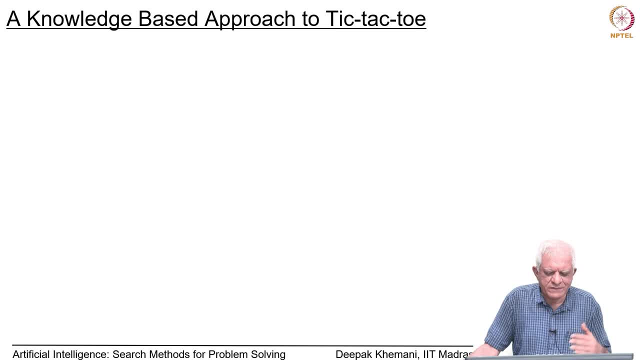 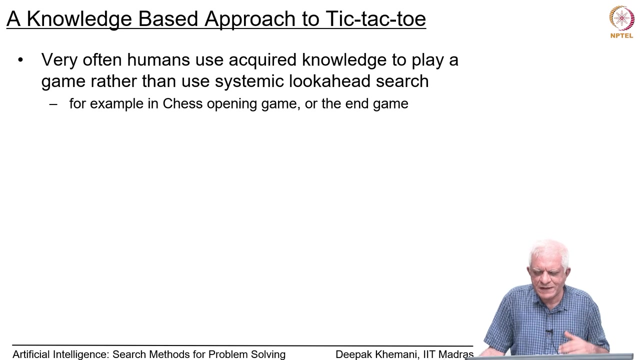 tac toe or any game, for example. we are talking about tic tac toe here, So we often acquire use, acquired knowledge. So, for example, if you are playing chess, then you might study a book like modern chess openings which tells you as to how the different openings are typically played. royal operas. 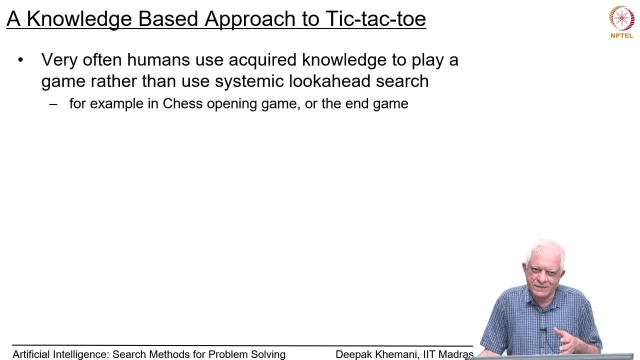 kings gambit, queens gambit or whatever the case may be, or the end game. you know, children learn that if you have two rooks and opponent has a lone king, how can you checkmate the opponent? You do not need to do search. once you have acquired that kind of knowledge, you can just 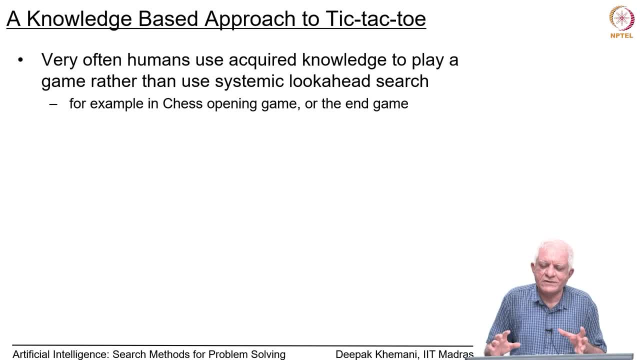 use the knowledge, and that is the whole trade off between knowledge and search. Search is good for problems which you have not encountered before. knowledge, if you have gleaned it from experience or from the experience of others, can be used to solve problems fast. essentially, 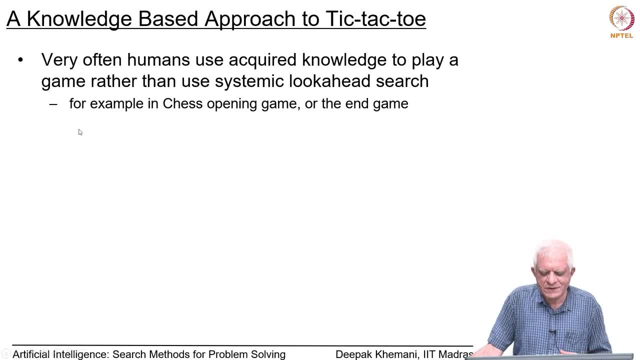 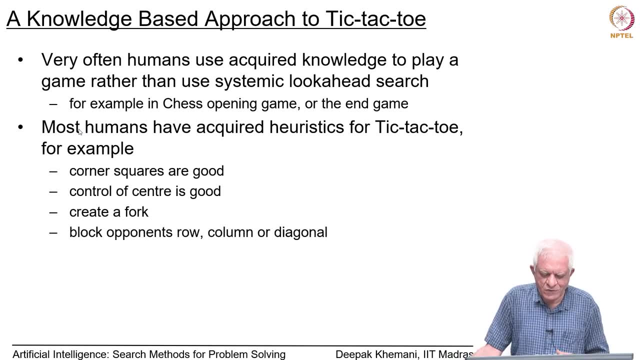 Search. of course, as we have seen throughout, this course tends to be exponential in nature, and very soon they figure out that the minimax value of the game is 0 and they also figure out how to play the game well. So, for example, they figure out rules like corner squares are good. center control of. 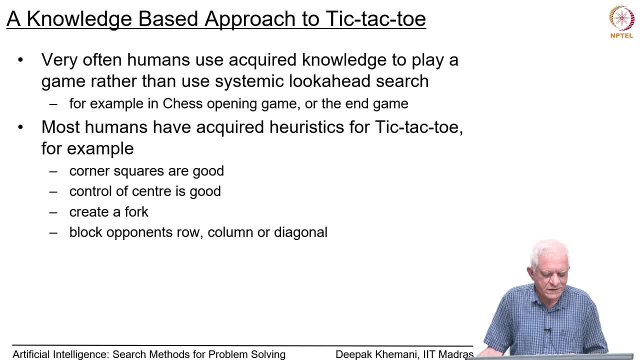 center is good. if you can create a fork, then you are likely to win, and you must block opponents from doing things like creating forks and winning diagonals. So you may use, build a vocabulary about which, in terms of which you can write rules. 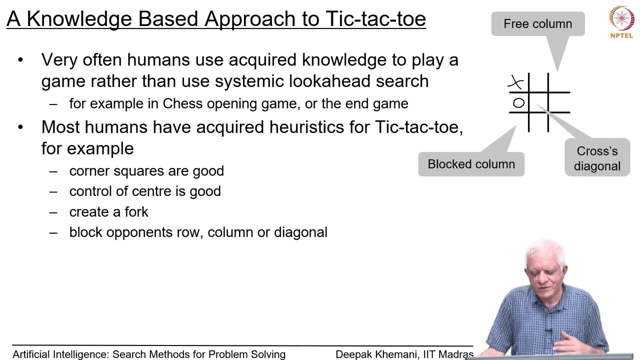 so you may identify free columns or a blocked column, or identify a diagonal which is available to a player, And then, as an exercise, I will leave it to you to try and write a rule based tic-tac-toe player, essentially. So, write them in an ops file language. you have to obviously invent the vocabulary. what 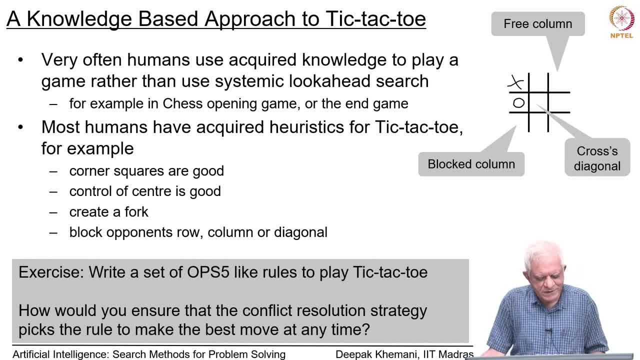 are the class names, what are the attribute names and so on, and also give some thought as to what should be the conflict resolution strategy So that your program plays. So remember that it is easy to play optimally in tic-tac-toe. 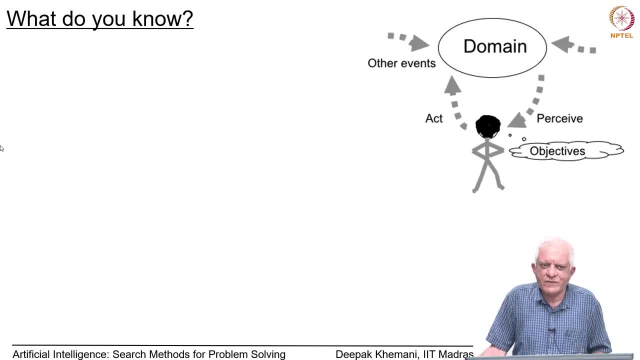 Now here is a preview of what is to come next week. When you look at an agent in a problem solving environment, and this diagram is something we saw when you are talking about planning a, an autonomous agent in some domain, operating in a dynamic world. . . . . . . . . . . . . . . . . . . . . . . . . . . . . . . . . . . . . . . . . . . . . . . . . . . . . . . . . . . . 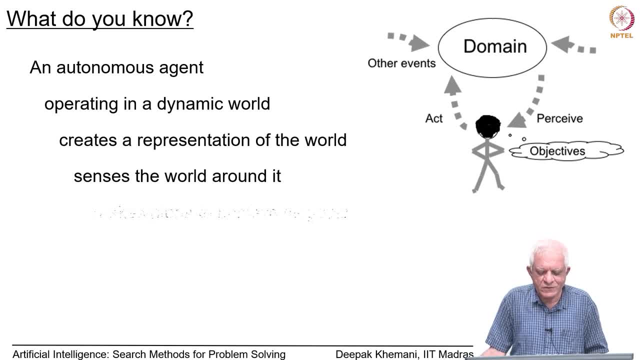 creates a representation of the world, senses the world around it, makes plans to achieve its goals, monitors the execution of those plans and constantly updates what it knows. So we are assuming a domain in which not only the agent is acting, but there may be 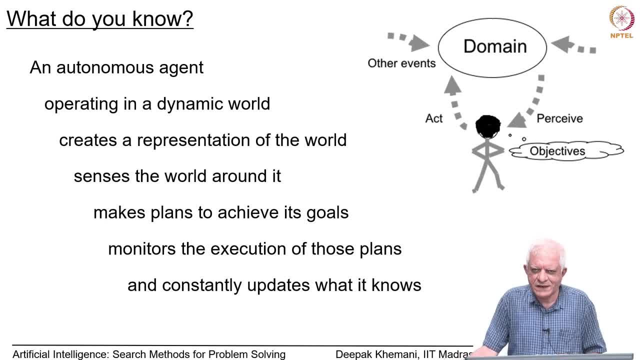 other actors as well, and that is why we are calling this a dynamic world. But in the real world, you will have to keep track of, be aware of what is happening around you, and that is an important part of being an intelligent agent. 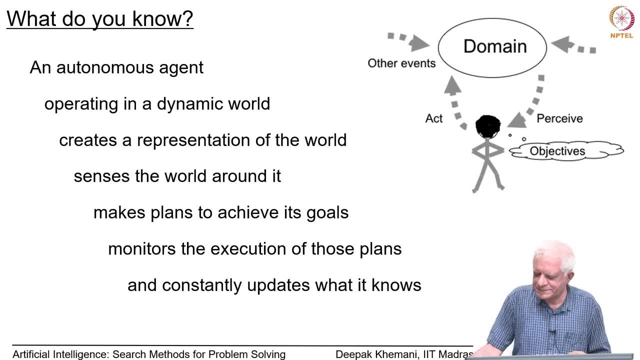 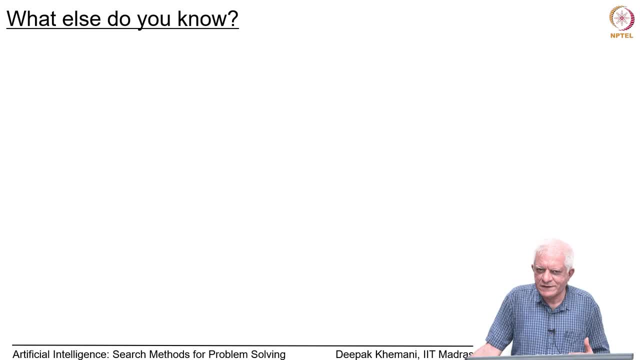 You have to create a representation of the world around you and keep updating it. So, apart from what you know about the world, what is also important is what else you know about the world, and we can express it as follows: Let an autonomous agent operating. 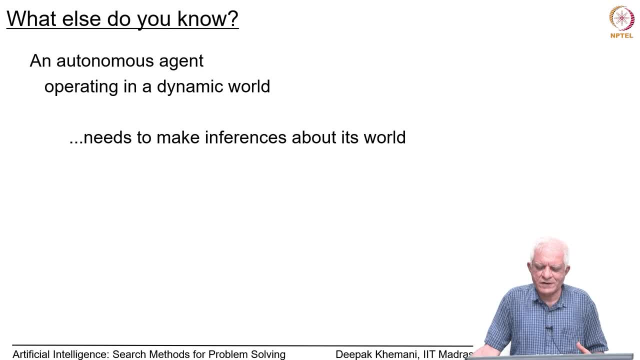 in the dynamic world needs to make inferences about its world. So you may see something, but based on what you see, you may infer something. essentially, That part of an agent's activity is what we will look at next. A little bit of logic about a week or so in this course. 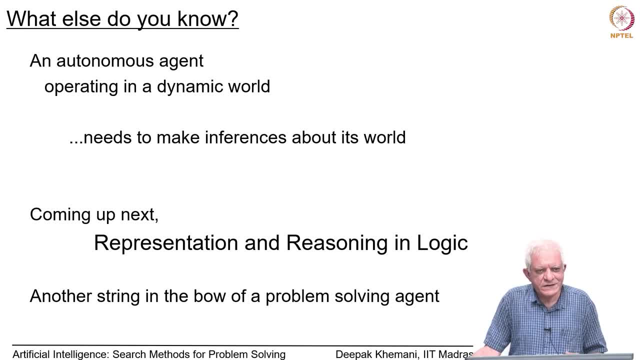 and we will talk about representation and reasoning in logic, which is another string in the bow of a problem-solving agent. So search is not the only way to solve problems. Memory serves a purpose. Memory serves a purpose of acquiring experience, remembering experience. 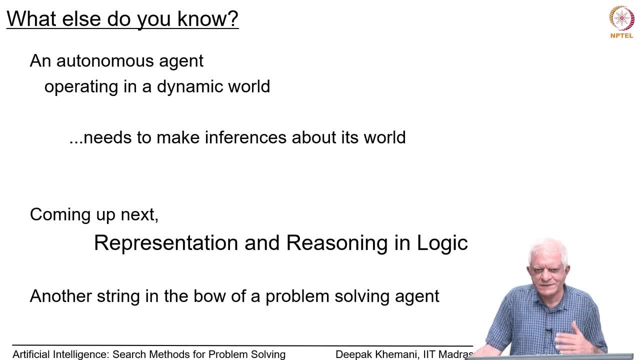 and there is a whole field called case-based reasoning or memory-based reasoning, which talks about how to remember things that worked in the past. But also from past experiences you can distill knowledge into the form of rules, and we have seen already that some 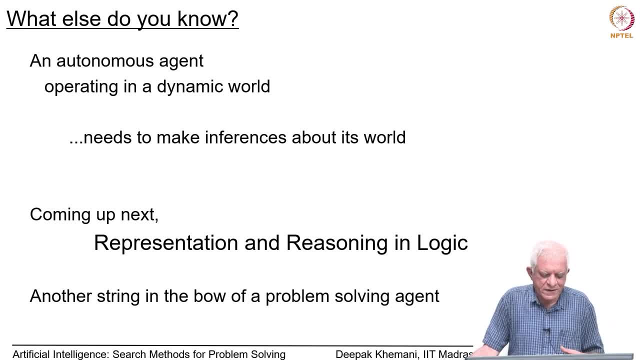 aspect of problem-solving, memory-solving, memory-solving, memory-solving, memory-solving and problem-solving can be done using only rules, But being able to make inferences is another critical part of being an intelligent agent, and we will spend the next week looking. at that, So we will see you next week.